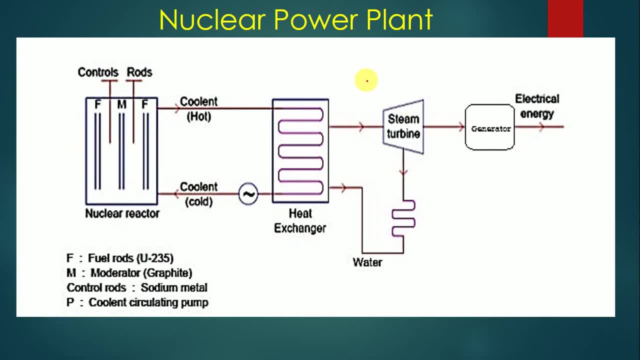 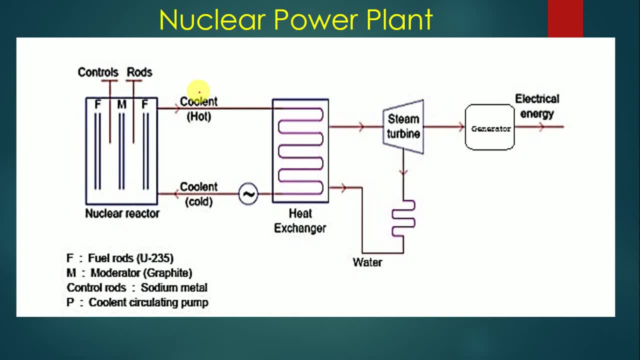 reactor for generation of the heat. that's the only difference, whereas the other working components are same. now let's see the construction which are available here. this particular part is called as heat exchanger, which was in the thermal power plant. it has called as a boiler, but now it is. 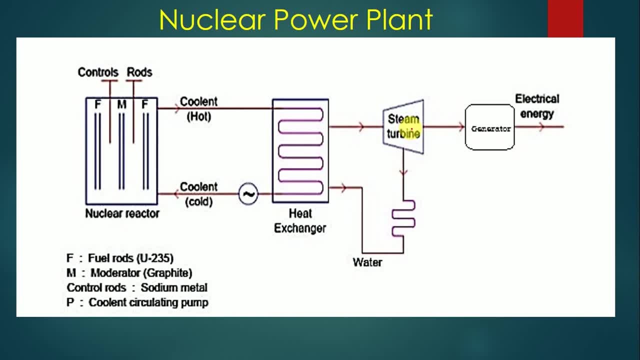 heat exchanger. this particular part is called as a steam turbine. this part indicate a condenser, this part indicate generator, and the heat generation system is nothing but a heat generator, nothing but this nuclear reactor. so this system is generating heat, which will give heat for generation of the steam. okay, so now let's see the various component. heat exchanger in heat. 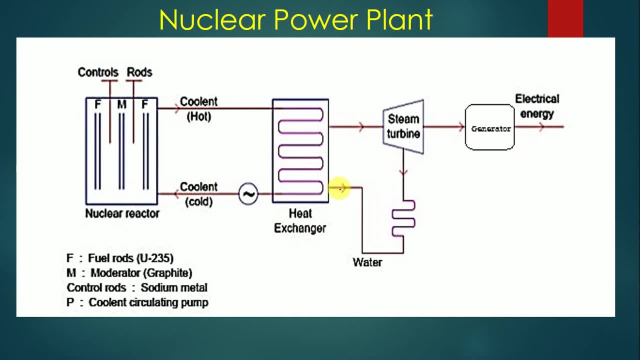 exchanger. here the arrow is something like this: with this we are giving cold water as inlet, so from this cold water will be inlet. this cold water will come in contact with this tube which we are observing. inside tube there will be heated fluid. there will be a heat exchanger which is coming from a nuclear reactor, so heated fluid is passing. 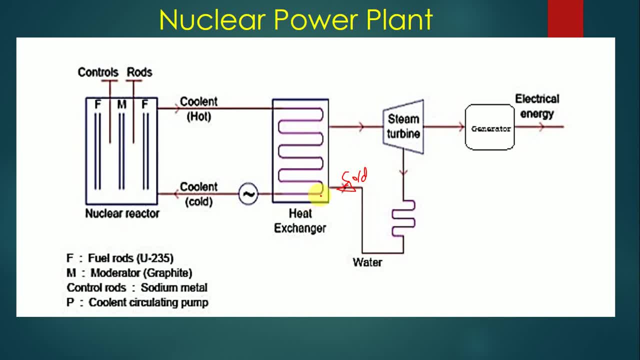 through this tube and outside of tube, what we are having is the cold water. so now there will be heat exchange between the tube tube fluid which is inside and the water which is outside of the tube. because of heat exchange, the water will get heated and one time will come that it will get convert. 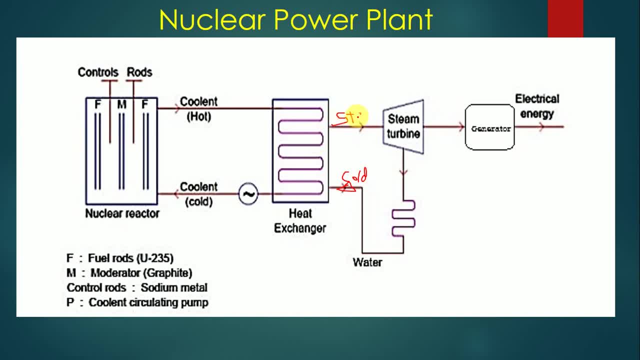 into the steam and at the output from this particular heat exchanger. we are having the steam as outlet- okay, applying as the input, and at the output we will. we will be getting a steam because of heat exchange. now this steam will enter into the steam turbine. this is steam turbine device in the steam turbine. 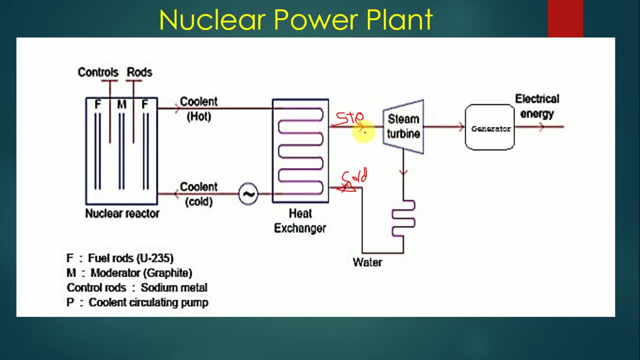 we will be having the blade and shaft arrangement. so when this steam goes inside it will give impact over the blade and blade start rotating and hence shaft will also start rotating. now when shaft is rotating means at the outlet of this particular steam turbine we are having mechanical energy. so 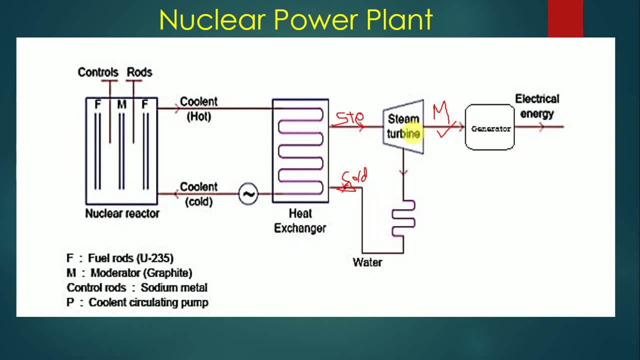 this is the output energy which is available here. this output energy will be given to the generator. now, what generator will do? generator will take mechanical energy as input and it will give output as an electrical energy. so here we are having electrical energy as the output, and that is what. 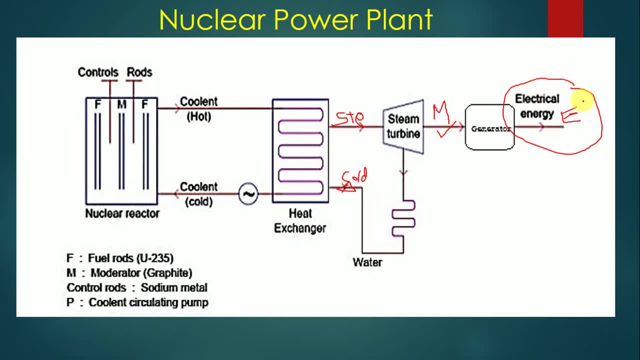 our total aim of this particular power plant where we get electrical energy as a output. so steam turbine converted steam energy into mechanical energy and mechanical energy get converted into electrical energy. you using generator, then steam which is coming outside here, that is low pressure steam that will enter 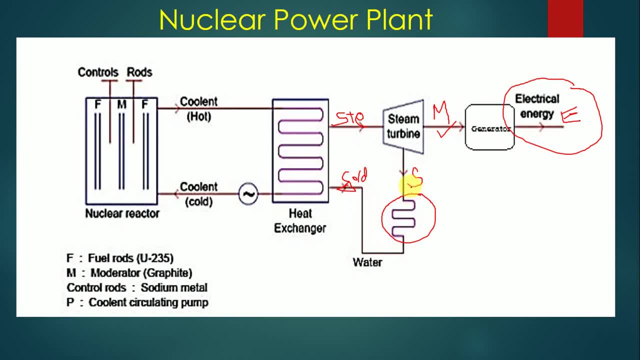 into the condenser. this particular device is called as condenser, so in the condenser the steam will get converted into water. that in condenser the condensation process occurs, means conversion of gaseous form into liquid form. so steam will get converted into water and that 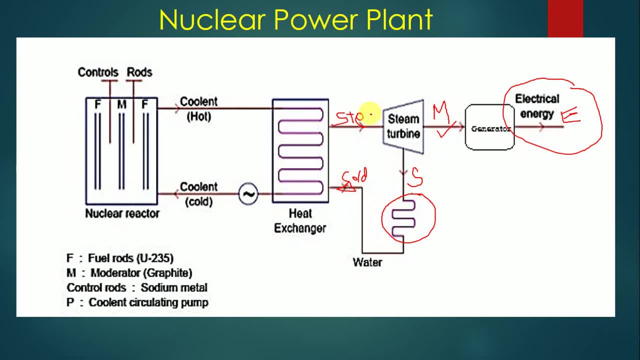 water will be again supplied. so this completes a cycle on the right side that the heat exchanger supplies the steam, steam goes to the steam turbine, produces mechanical energy and that steam comes outside that goes to the condenser. in condenser, steam will get converted into water. 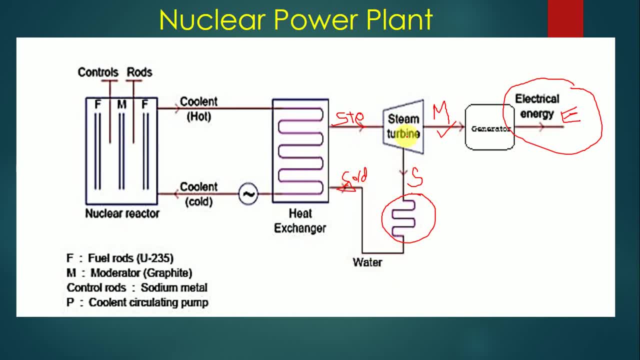 and that water again is supplied. so this cycle will go on continuously. okay, so this cycle is very similar to thermal power plant. so, coming to this particular system, that is what nuclear reactor and how heat is generated. okay, so let's see how it will be working here. now let's look at an example. okay, this is a nuclear reactor. okay, if you see nuclear reactor, 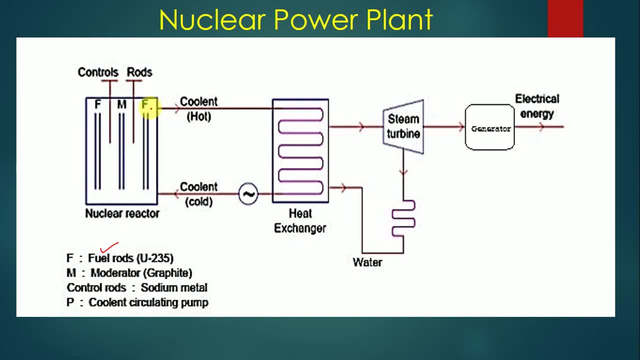 there are three alphabets. we have used f, m, f. f indicates fuel rod, m indicates moderator, and again, f is what fuel rod. there are also a control rod and the control rod used as a sodium meter. okay, so here, the fuel rod which we are going to use is the uranium. so uranium is used as a fuel and because 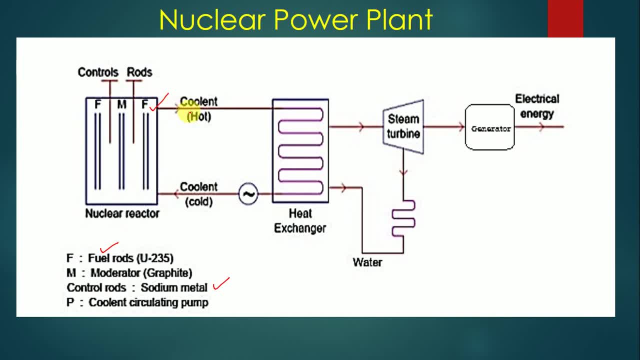 will be heat generation. because of that heat generation, the fluid which is available that will be get heated and that heated fluid will come into the heat exchanger. that heated fluid lose its heat to water, water get converted into steam and steam goes to the steam turbine. okay, 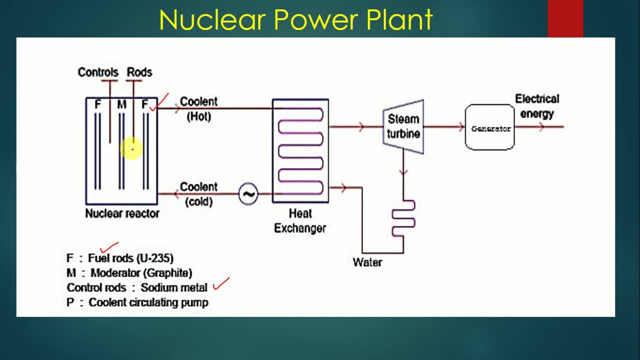 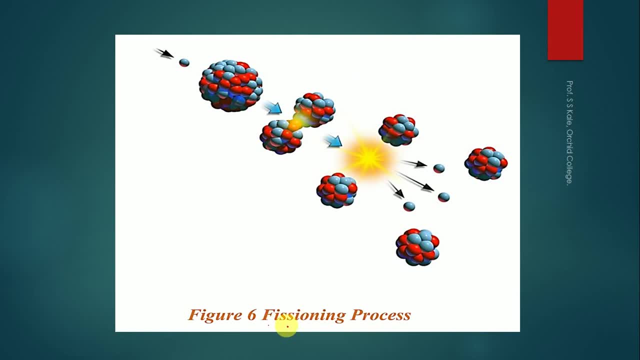 so, because of reaction occurring in a nuclear reactor, there will be generation of the heat. now, what is reaction occurring in the nuclear reactor that we have to check? so this is particular process, that is what called as fissioning process, by using which the heat is generated. here the 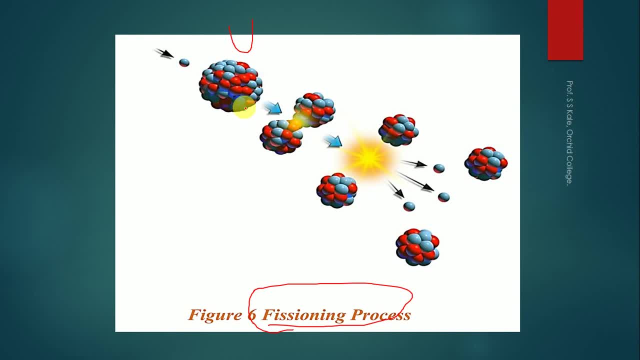 fissioning process is shown. let's consider that this is uranium fuel, uranium fuel and this is a neutron. so when neutron bombards on the uranium, the uranium will get will get split. so here you can see that uranium gets split into two part, and when it will get split into two part, there is a 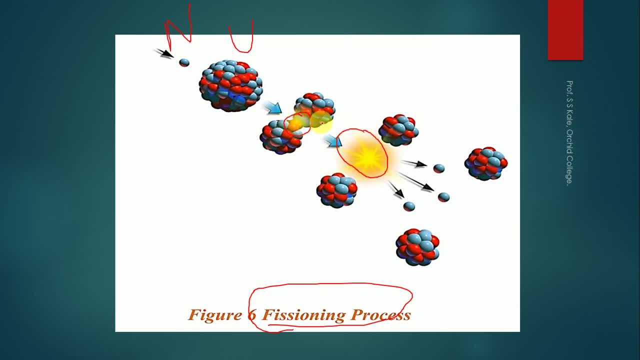 generation of heat. you can check here that there is a generation of heat. so when the splitting of the electron occur, there is a generation of heat. when splitting occurs, the neutrons also get split. so here you can see that neutrons are also get split and by using these 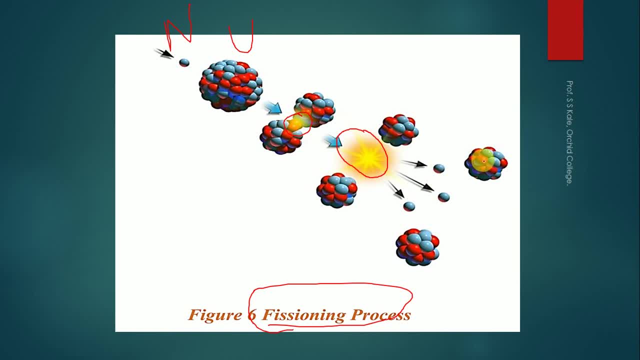 neutron, again, further splitting of the uranium will occur, like if you check this particular neutron, this neutron will bombard on this particular fuel or uranium. this will again get split. when there is a splitting again there will be generation of heat, like that chain reaction occurs. like that chain reaction occurs. 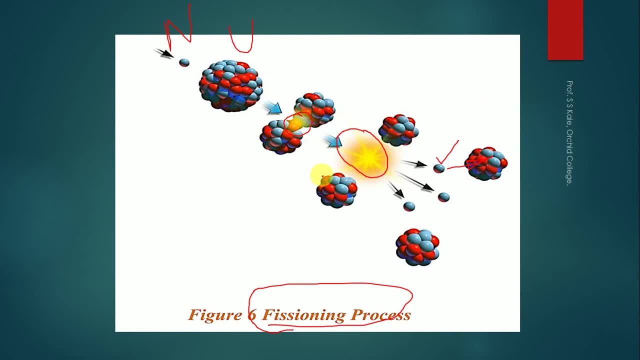 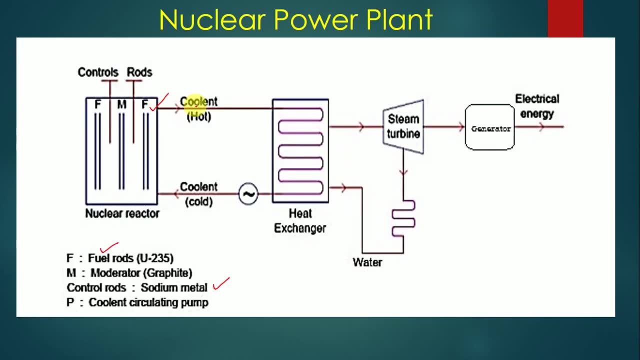 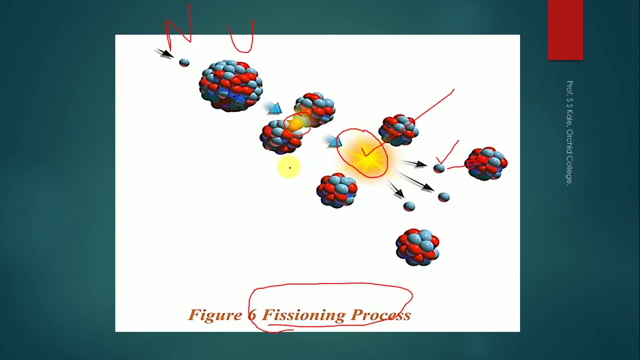 and because of this chain reaction, what is happening is the heat is generated. okay, so by using this particular heat, we are going to heat and fluid which is present and which is circulated through this particular tube and that is used for converting water into the steam. so this particular 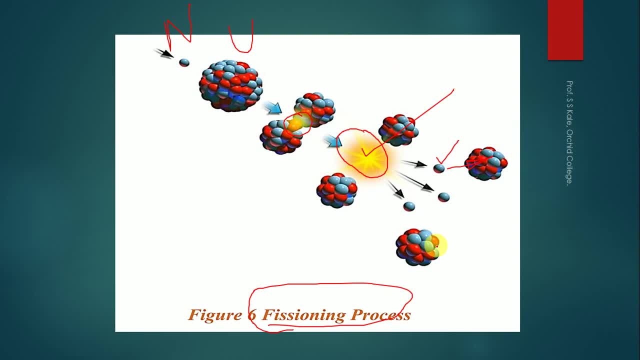 process is called as a fissioning process, in which heat is generated, and it's a chain reaction. you have to remember that the uranium which we are using here, that will get split into two parts. so let me unsere the earth, forgive this vision if you have seen that they have completely collapsed. 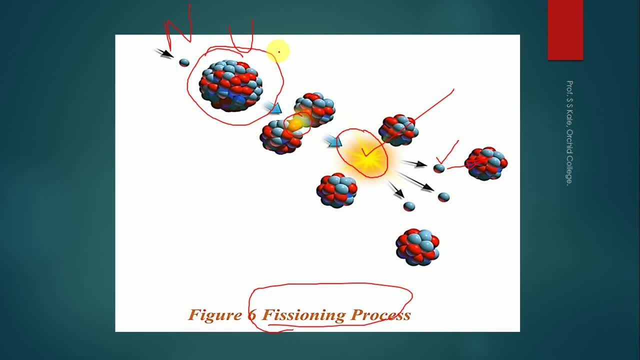 and theyocked and either were filled by a turbine or 느� gå pe trap structure. do not to worry, it will all be angle printed with one coloredừa. it is a thin copper, so this, printed and housed, ensure that we have enough area for the heat nownah, and.